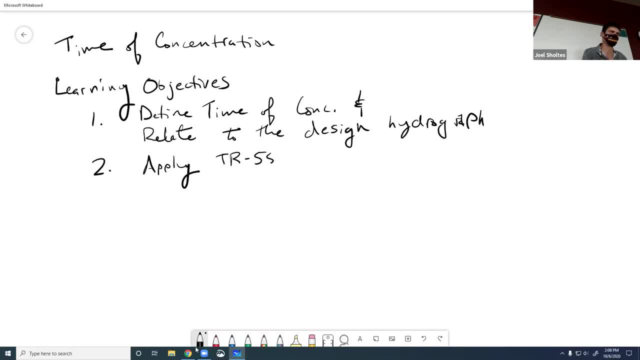 We will then apply- I'm going to call it TR55.. There's, it's really kind of a compilation of methods, but I'll call it the TR55 method- to estimate time of concentration. So, for example, we can just introduce and apply. 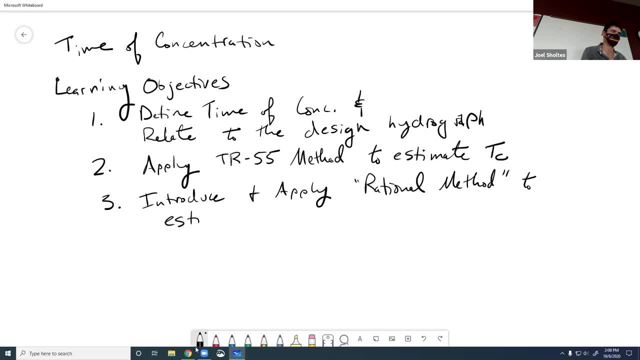 the what's called a rational method to estimate peak discharge. It's kind of like a quick and dirty way to get a peak discharge- The TR55 method. we're not. we're not quite there to get peak discharge. We'll focusing on the TR55 method. 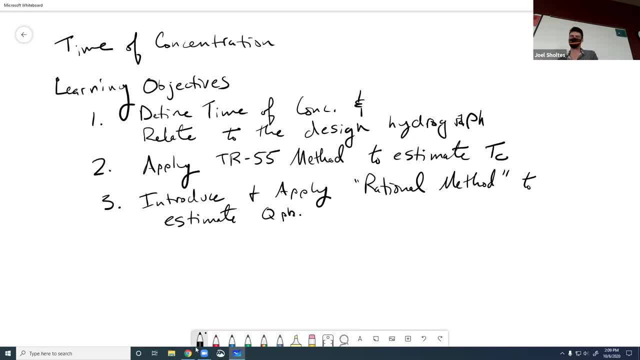 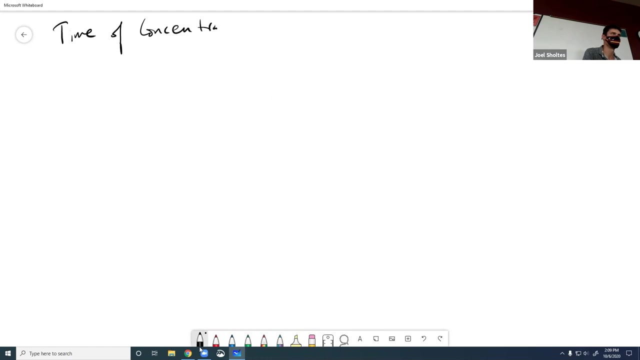 finish that journey on Thursday. Okay, So we defined time of concentration right, It is TC right And this is the time required for the most. we'll call it hydraulically: distance point in the watershed to the outlet, I should say the time required for water to 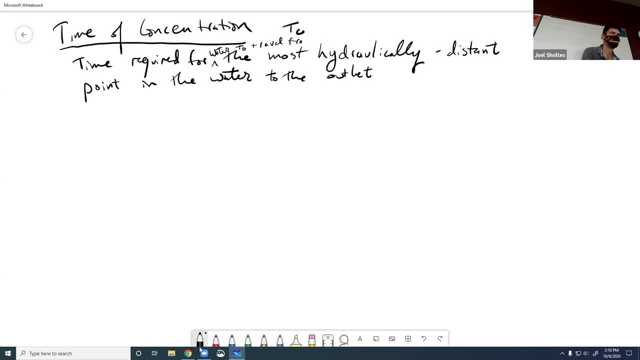 travel from the outlet is a runoff right, Also known as the longest travel time. Not necessarily the longest distance, but the longest distance is going to get us close enough, So we'll just kind of take a look at that. Here's a funky watershed. 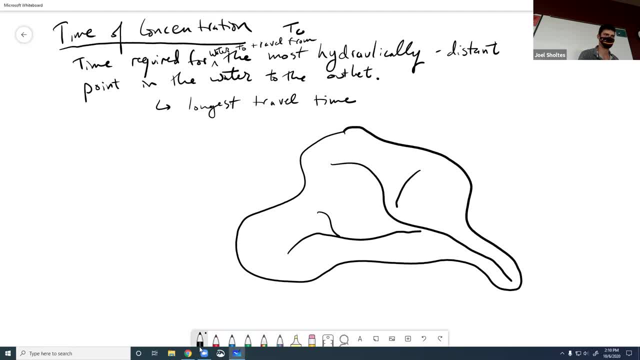 Okay, You can tell me what order this watershed is, if you're like a stream water. Do you guys remember that? 1. So this would be 2, right? Two 1's come together, we get 2.. 1, 1. That's 2.. So two 2's come together, we get a three. 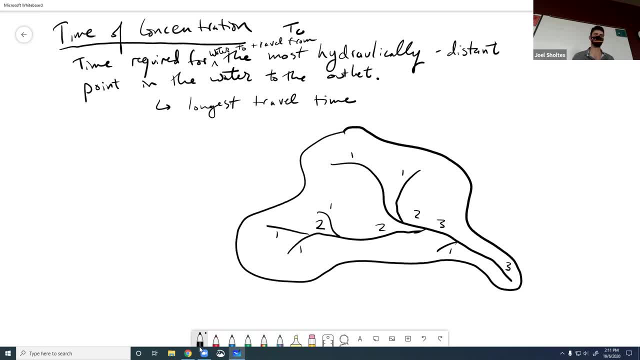 Okay, just a little practice. We'll keep practicing that Third order watershed, All right, and we want to think about the water droplet coming from the most hydraulically distant, So we'll pick here. This looks like it's the farthest, So it falls on this ridge and then it travels as 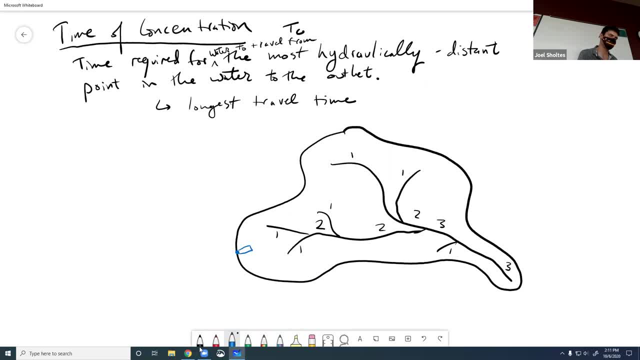 sheet flow- We'll define these in a minute- So kind of shallow sheet flow, and then it kind of for a certain distance and it becomes- I'll call that sheet, and then it becomes shallow, concentrated flow, kind of like rills. It eventually hits a channel and then, once it, 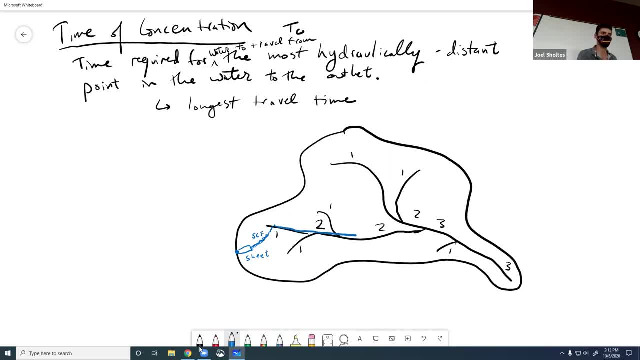 hits that channel. we're kind of zooming. We're going pretty fast all the way down to the outlet. So our time of concentration is going to be the time it takes to travel all these three-dimensional flows. So we're going to be traveling all these three-dimensional flows. 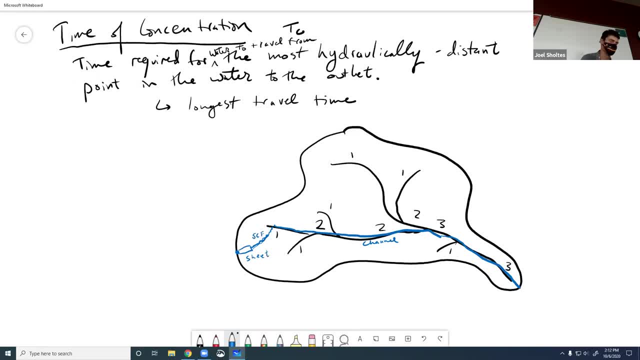 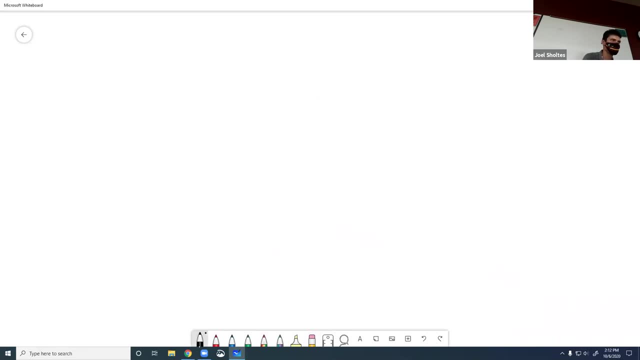 So we're going to be traveling all these three-dimensional flows, So we're going to be three different routes, and that's kind of a simplification. but it's how this method works. We think about it as three different routes And our time of concentration is going to equal to. 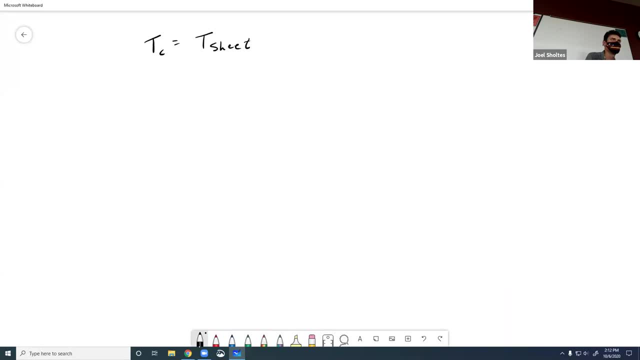 the time we spend in sheet flow, plus the time we spend in shallow concentrated flow, Plus the time we spend in the channel. We need to estimate these and then add them up and we get our time of concentration. But then how does that time of concentration translate to an actual hydrograph? How do we? 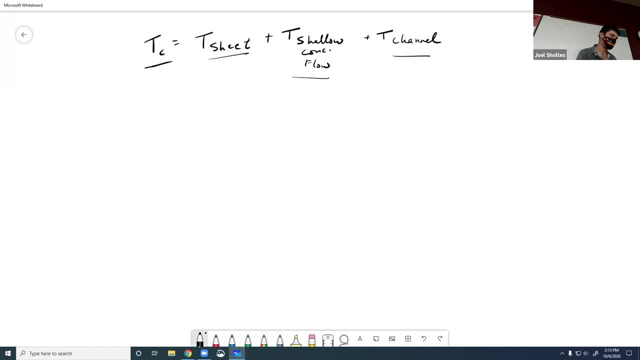 relate this to the hydrograph. Well, let's look at that. So here's a hydrograph. Usually they kind of do it like this. So here's a hydrograph. Usually they kind of do it like this. So here's a hydrograph. 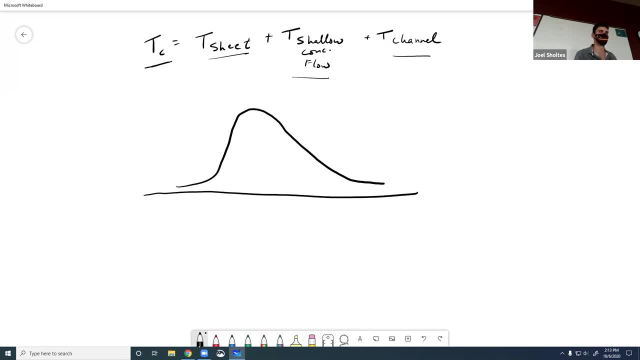 So here's a hydrograph. So they kind of come up quick and then they might tail off, So they might have like a longer tail than on the front side. That's our hydrograph, So we'll have time over here. We have discharge over here. 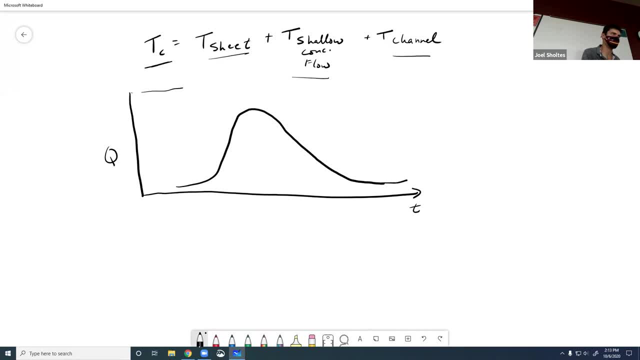 Then we're also going to represent the hydrograph. I'll just keep it simple and just make it one little point: input of rain, And so this is going to be our precipitation depth in inches. So we just get some unit of rain that comes out. 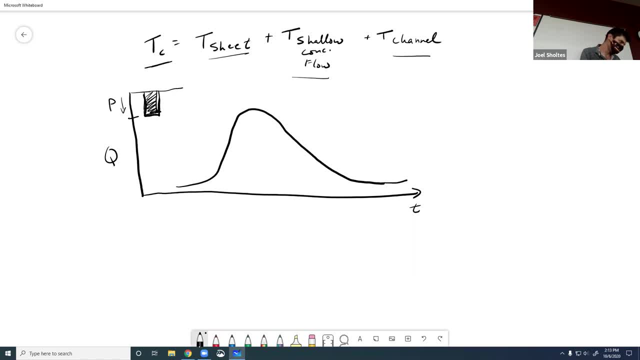 And let's think about how we model rainfall runoff. You guys are working on your HMS models right now. You've created your design storms right, You've estimated the rainfall depth associated with a certain frequency storm And you've done all these little adjustments based. 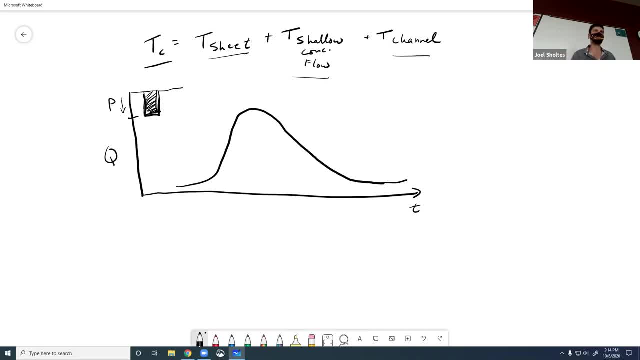 on the point to area factor and the time distribution, right. So you've created a hydrograph, That's your kind of design storm. So that's really all we know. We don't know. We're kind of: that's our input, That's our 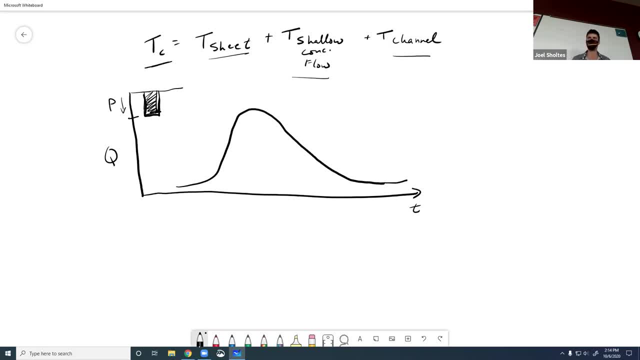 that's the one thing we know. And then the other things we know are the properties of our watershed, right? You know the area, the slope. you're going to estimate some of these parameters, the curve number, that sort of thing. So what rainfall runoff modeling does is it takes this: 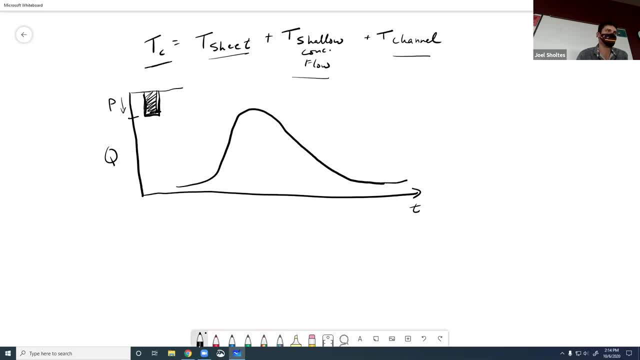 rainfall input and it translates it into an outlet hydrograph. And what this time of concentration calculation does is it tells you. this is basically. this one number summarizes the properties of your watershed. How long is water going to spend in the creek? How long is it going to spend on some hill slope before it hits the channel? And so that one number 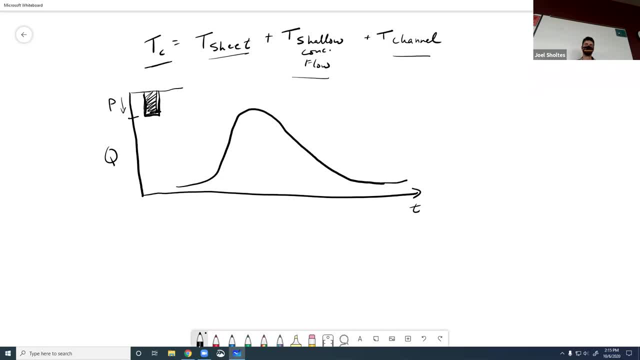 besides the area and the curve number describes the kind of hydraulic properties of your watershed by all these flow percolations has. And what it does is it tells us the relationship between when that rainfall comes in and when we get this peak of the hydrograph, And this is the lag time. So it's the middle, the kind. 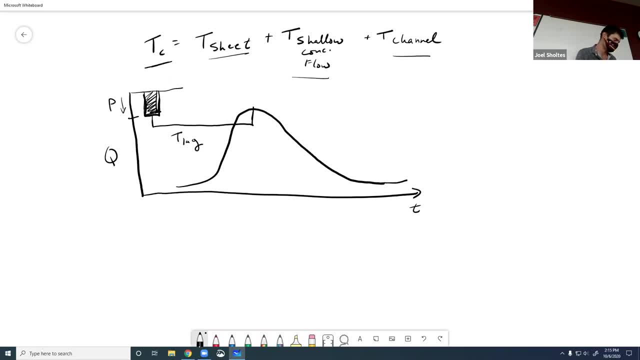 of centroid of your rainfall to the peak of your hydrograph. And then if we look at the point of inflection on a hydrograph where we go from concave- this isn't a perfect drawing here, but if we go from convex to concave we have some point of inflection where that. 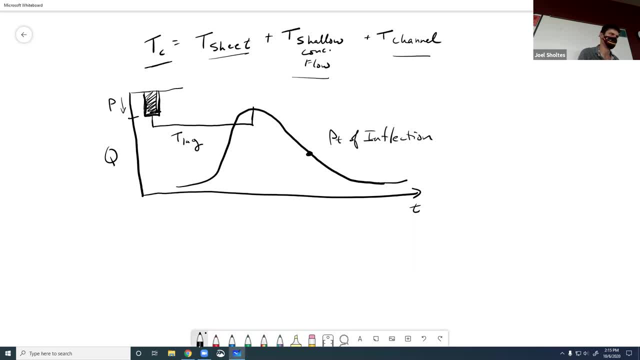 curve changes. That is going to be our time of concentration between that rainfall event and that point of inflection. This is kind of some theoretical thing, right, And we talked about time of concentration would be a hydrograph that has a. you have a steady input of rainfall. a hydrograph comes up and then 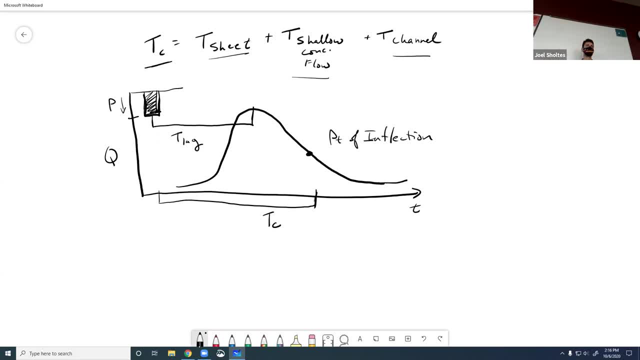 it flattens out because everything's in equilibrium: What's coming in is equal to what's going out, and you get that flat hydrograph. So we're never going to really see that. That's kind of a theoretical thing, So people relate it to the point. 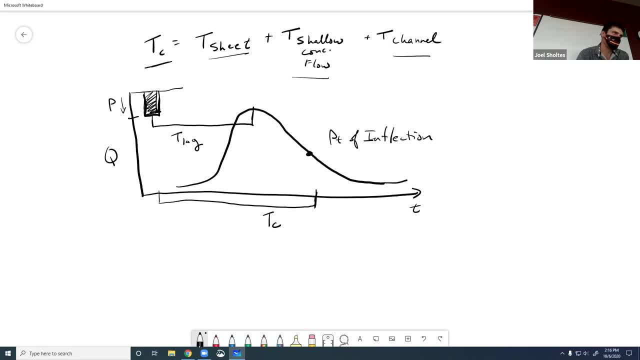 of inflection And the kind of rule of thumb. how do you get to? what is the point? inflection? That's not really a super useful thing to know, and so we take a step to relate the lag time to the time of concentration, And this is: 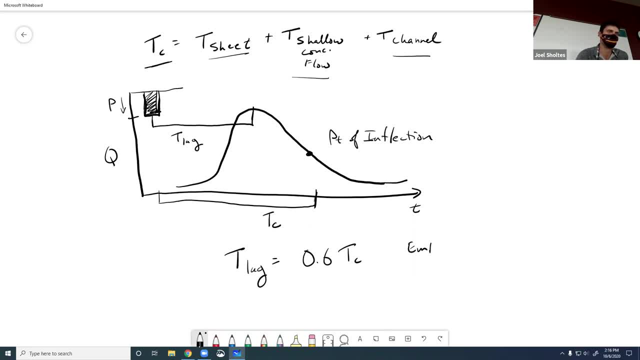 just kind of an empirical rule And the idea is we're not going to know the lag time ahead of time, but we can calculate the time of concentration based on that hydraulically distant point and relate it back to the lag time to the 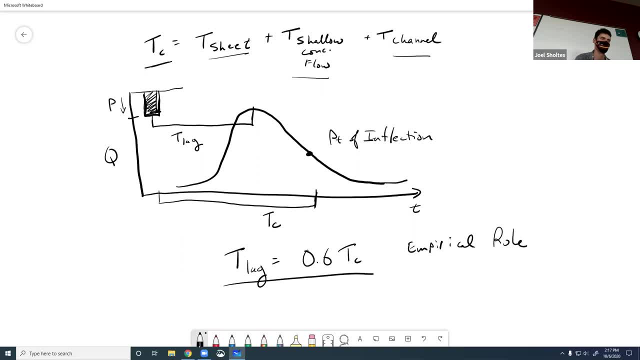 peak this time to peak right here via this relationship. So that's where we're headed with this. All right, so I'm going to keep this water shut up here. I'll simplify it. Every time I draw a water shut, I'm going to go back and see if I can get. 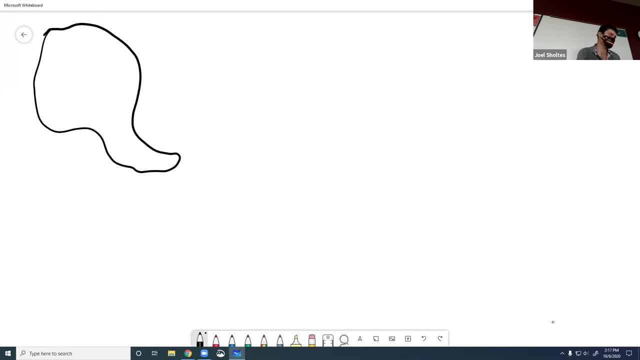 I'm worried I'm going to draw something weird scene, I don't know. So here it is. Here's our watershed. It's a simple one And we will focus first on- I'll make this red. We'll first focus on sheet flow. 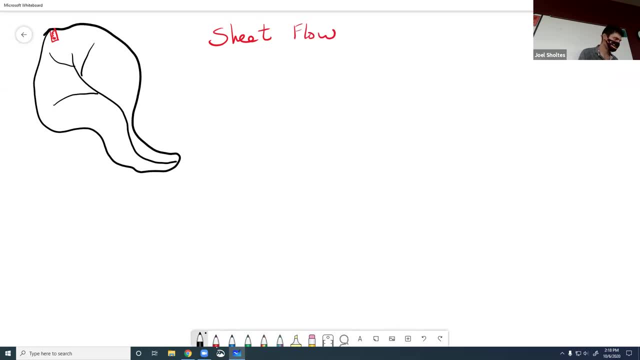 Remember, sheet flow is that real kind of just sheet of water. It's really shallow And obviously you can see it on like a parking lot. if it rains really hard You could probably see it in the deserts. You're not really going to see this on a grassy area, forested area. 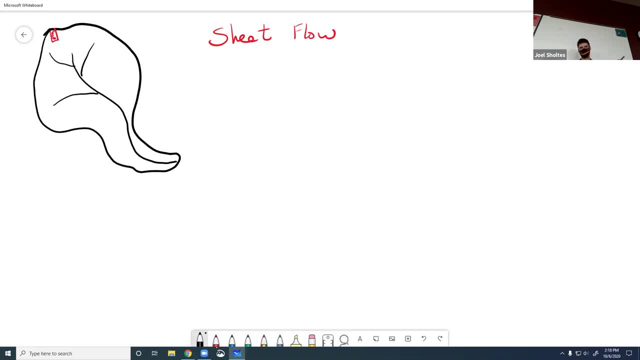 It might not even exist in that kind of setting. So, at the end of the day, this is, you know, an estimate, and we're just we're going to use it to kind of roughly estimate how long it takes water to go across the land. So the first thing about sheet flow we need to know is that we only apply it to the first. 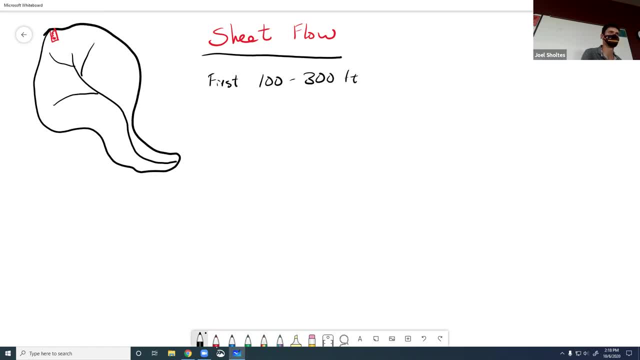 100 to 300 feet of flow. 100 would be for a steep situation, 300 would be the maximum for a we'll just say, mild slope, hill, slope. What's steep, what's mild. There's just a rules of thumb and you can take a look at the guidance document for that. 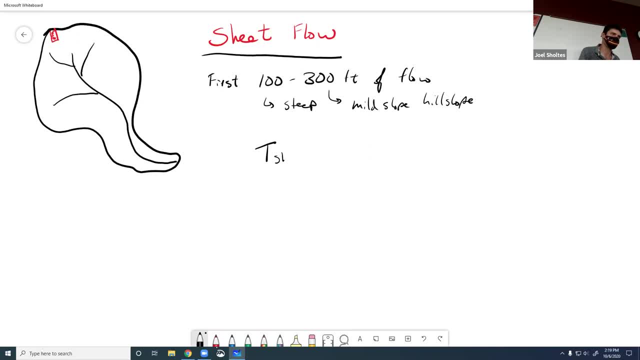 And we have an equation we'll use as an empirical equation, like most of this is So: time to sheet. time of sheet flow in hours is equal to 0.007 N times L. We'll define those in a second: P2 to 0.5. 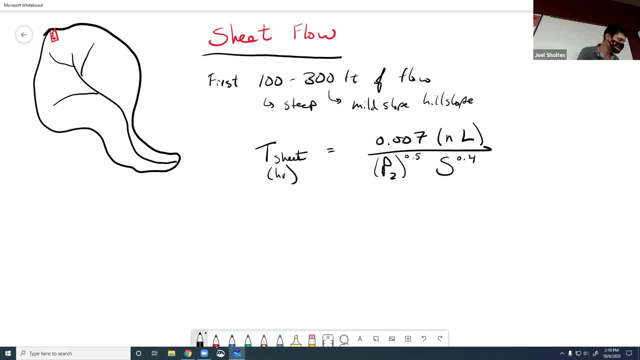 S to 0.4.. So very clunky empirical equation. Let's take a look at what these are. Does anyone recognize N? I'll give you a hint. We learned it in hydraulics, Manning's N. So Manning's N, remember. this is the roughness coefficient. 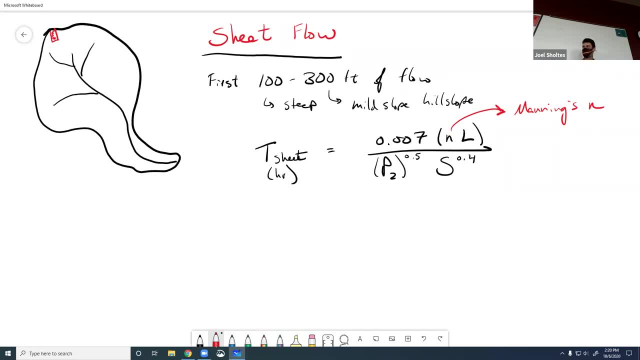 The higher the number is, the rougher the surface water is traveling over is, And so Manning's N could equal anything from 0.01 for pavement All the way up to 0.8 for, like dense grass brush. So a bigger number up here in the numerator is going to mean a longer time of flow, right? So rougher slows water down, longer time. 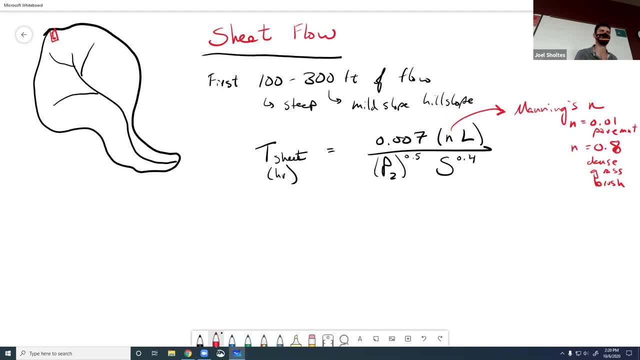 L is our length of the flow path in feet, S is our slope in feet per feet. And so just as long as it's just a percentage or a fraction, And then not a percentage or fraction, And then P2 is the 50%. 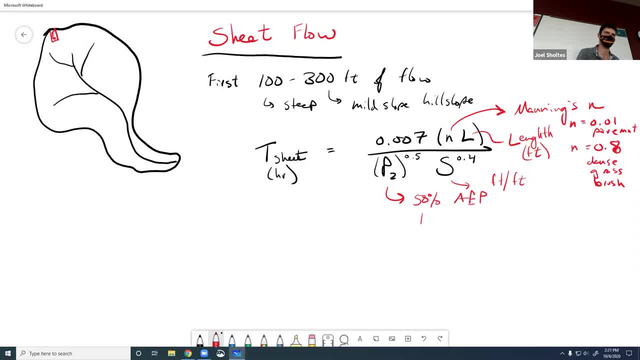 AEP: rainfall depth in inches. I love these non-homogeneous unit equations, But that's hydrology- for you At least engineering hydrology, I should say So it's a weird equation. There's a lot of different things we have to calculate. 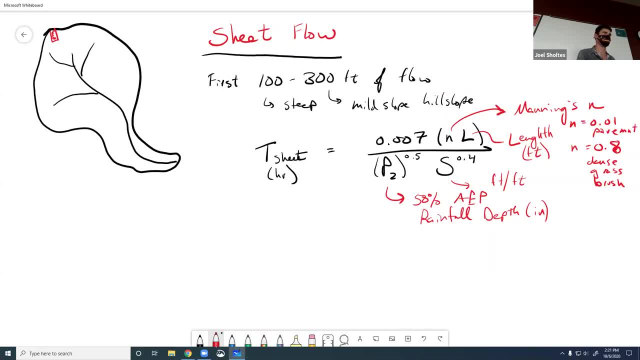 So you can imagine, and we'll actually do this, And for this lab is to go, you'll say, okay, I think it's a pretty steep slope, So I'm just going to do the first hundred feet, All right. so that's our L. 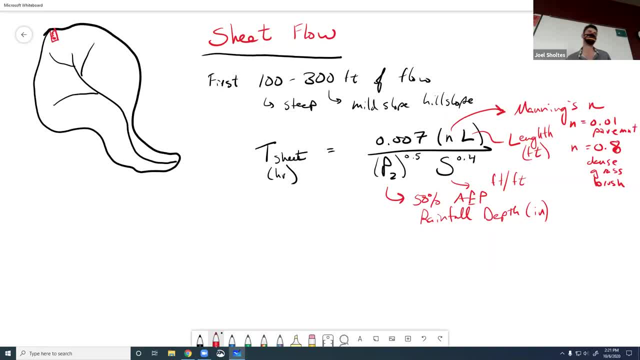 I'll look at the ground cover. Maybe you go out and walk it in the field. Is it pavement? Is it grass? There's a table here And that table is Table 15.1.. You can take a look at that. 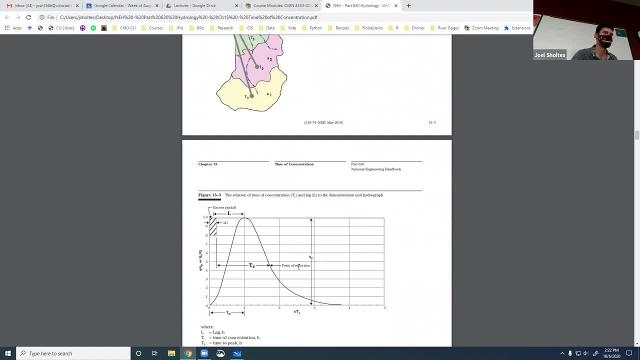 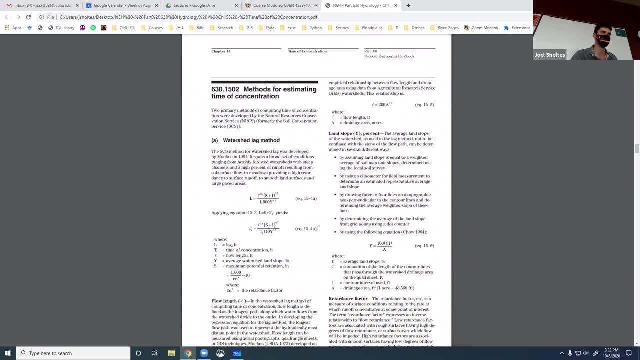 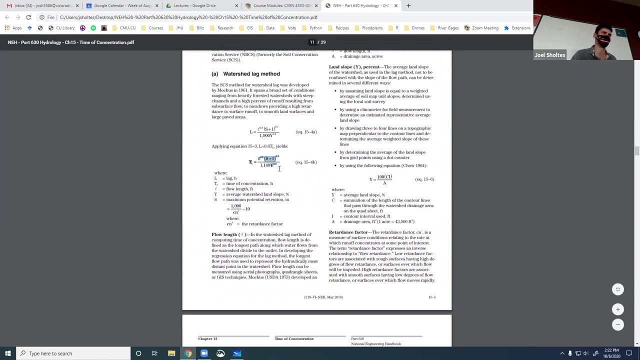 Here's a nice little definition of time and concentration. Here's that hydrograph And There's different methods in here. I'll tell you right now like this equation just gives it to you, the time of concentration All at once, based on some stuff. 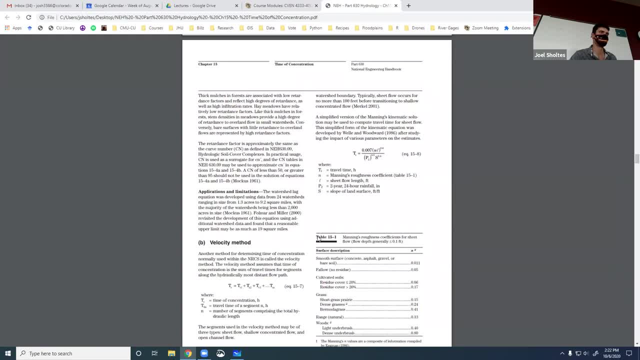 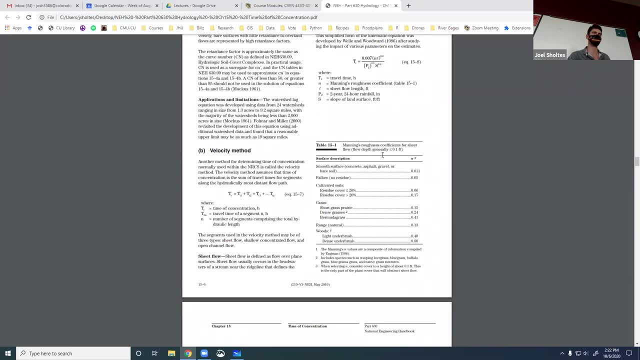 So you could compare. I might have you guys compare, All right, 15.1.. Here it is Manning's roughness coefficient for sheet flow less than a tenth of a foot depth And they give a smooth surface like concrete asphalt. We have different fields, different grass types, range, woodlands, 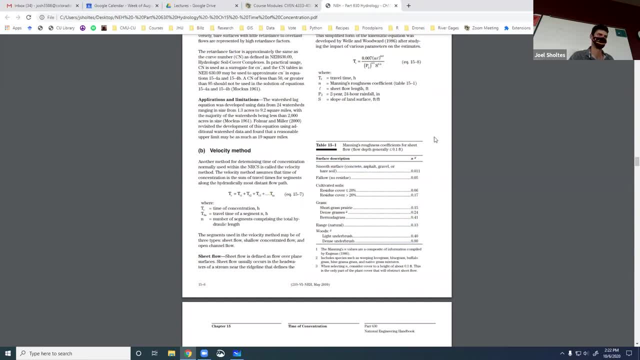 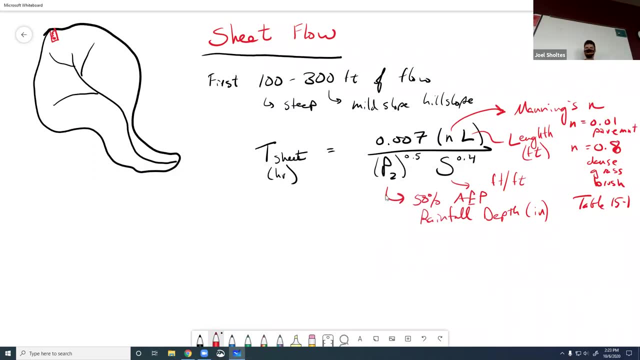 So that's our range of Manning's n values right there. And then where would we get this 50% AEP rainfall depth from? So NOAA Atlas 14,. we could do that Or we could stream stats. In Colorado they calculate all this stuff for you. 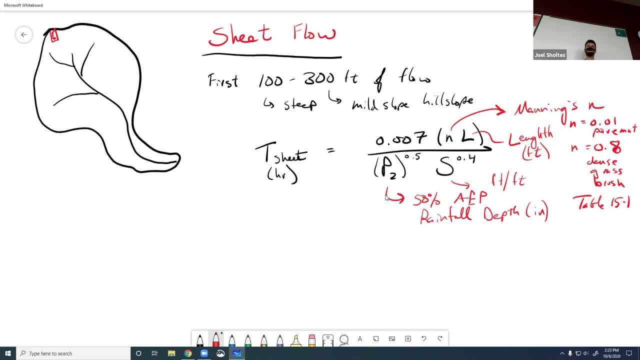 Because behind stream stats in Colorado they actually do this curve number method, the NRCS TR55 thing. So they'll calculate that for you too And then slope- you know, dy over dx. right, They calculate every flow time, They will just pick the most distant one. 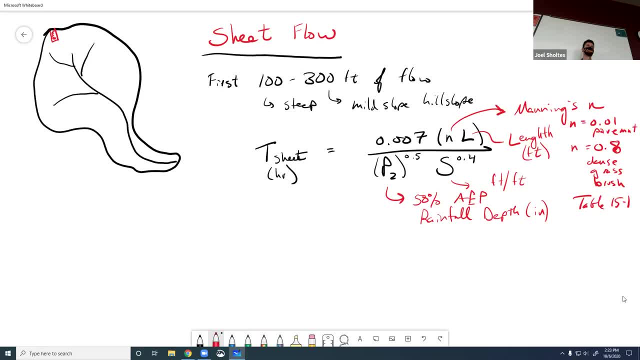 I don't know how that works. Yeah, I don't know how that works. Yeah, I haven't looked into how you automate it because there's a little bit of a user, you know, artistic part of this thing. So, yeah, there's a lot of assumptions that I'll have to go into it. 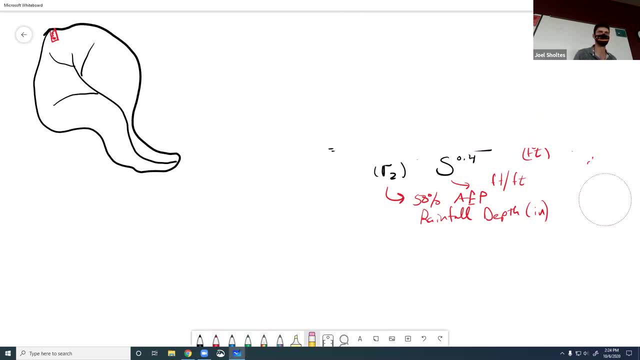 All right, that's sheet flow. Now let's do Shallow concentrated flow. And how am I tracing this line right here? Obviously, I don't have any information, But when we do this together, we'll look at contours and water is going to flow perpendicular to those contours. 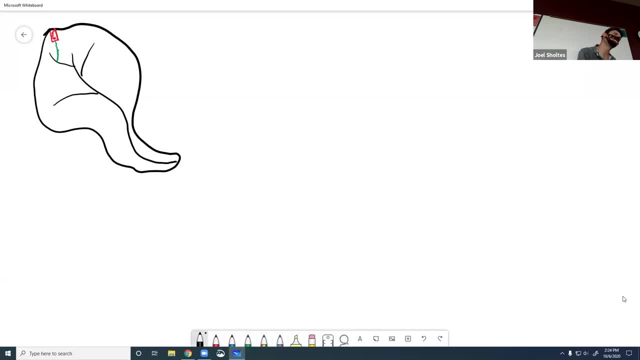 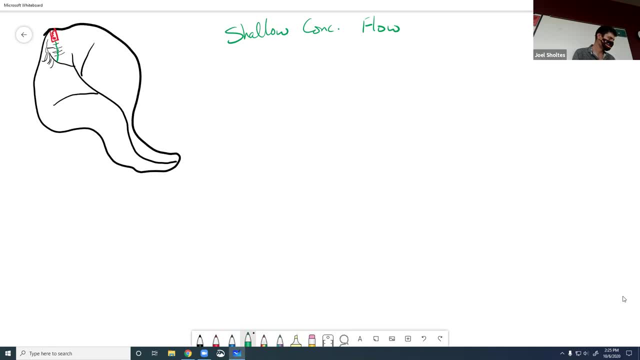 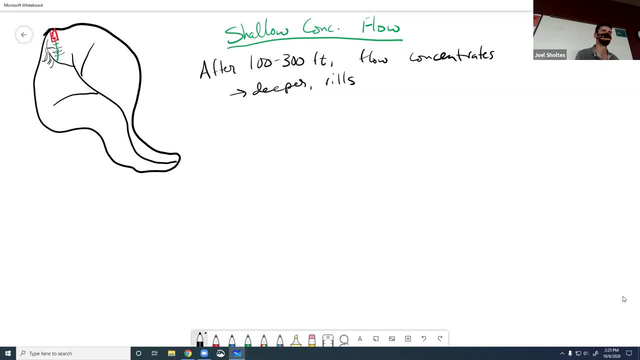 And the deeper water gets, the faster it moves. So this is going to be a shorter time. and the way we calculate Shallow concentrated flow again in hours. So we'll start with length: Over 3600 Times V. Right, So this is just a unit conversion thing. we're taking a velocity. 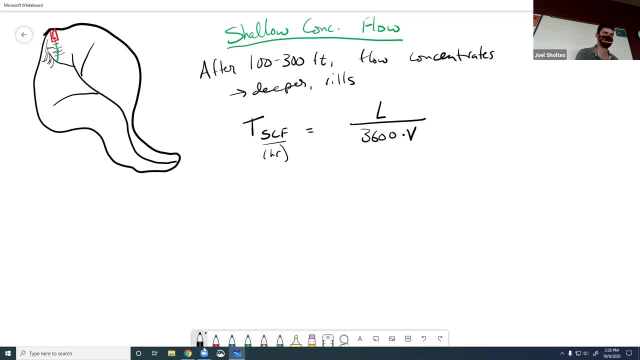 And we are converting it to a time Feet and feet per second. but we need to calculate this velocity. What is that going to be? So we'll go to a nice table and we've got some empirical equations. Again, this is based on Manning's and we say: velocity is equal to some coefficient which we can look up. 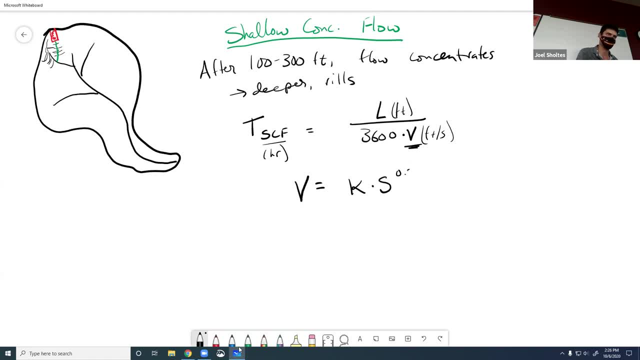 Times S Our Slope to the 0.5 and you'll recognize this part from Manning's equation. So all of this is kind of simplified. Manning's equation and S again is in feet per feet or meters per meters, And we want to look at table. 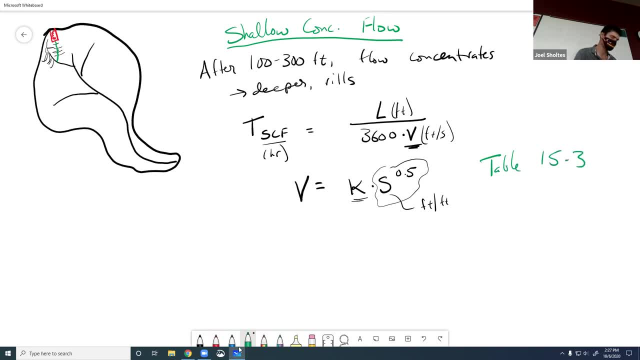 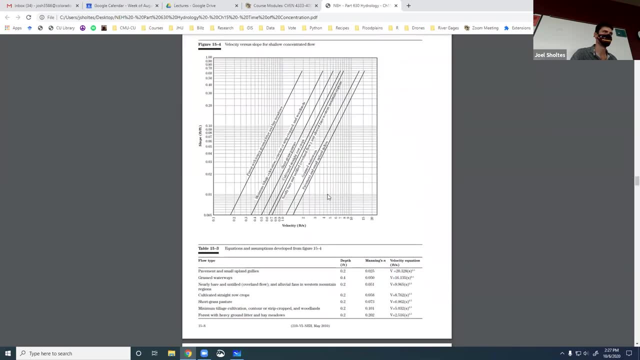 15, dash three. So let's take a look at that. So what this is showing you is just a very simple equation. It's this power law equation where you have velocity down here, slope up here. I might flip this if I were really. 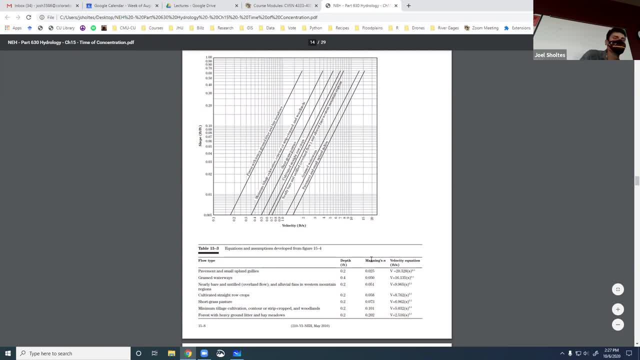 Because you know, velocity is our dependent variable and slips the independent variable. but it shows you that you've got different kind of covers: forest with heavy ground, litter, pavement, down here, somewhere in between, We've got, you know, grass, pasture. It assumes some kind of depth for those. We're not going to know what that depth is. it assumes a Manning's roughness for those different land covers and then it gives you this coefficient, So that K coefficient is going to be this number right here. 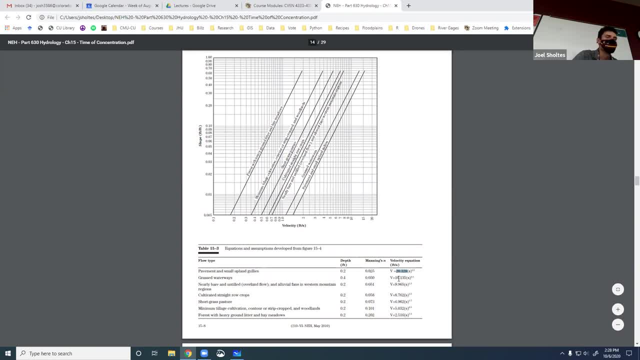 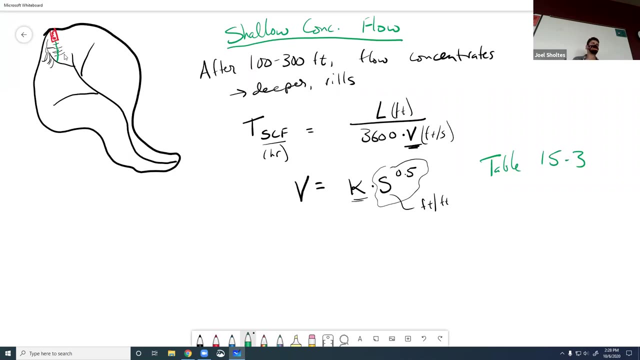 Or you could use this figure. Either way, it's not a, it's not a very hard equation to put a number into. So, yes, to make your slope along that line Pathway. and how do I know where I start and stop? Well, I need to see a channel there, and maybe that's something I found in the field, Maybe it's something I can see from aerial images, or maybe it's like a blue line that USGS has drawn on their, their topo map. they've identified this as a channel. 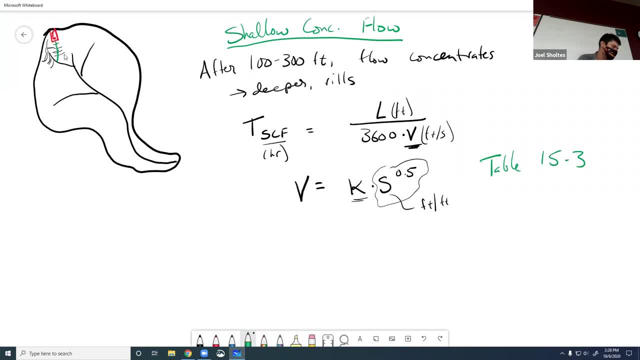 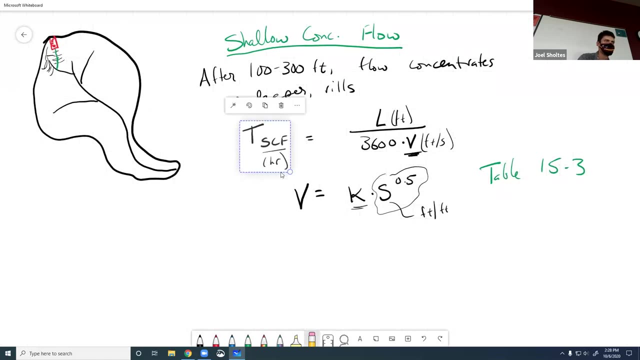 So that's going to give me my length and my slow, based on the change in elevation between those two, And so that's going to give me a Catalunya for that. Okay, This is getting complicated, Alright. last stab, where we at 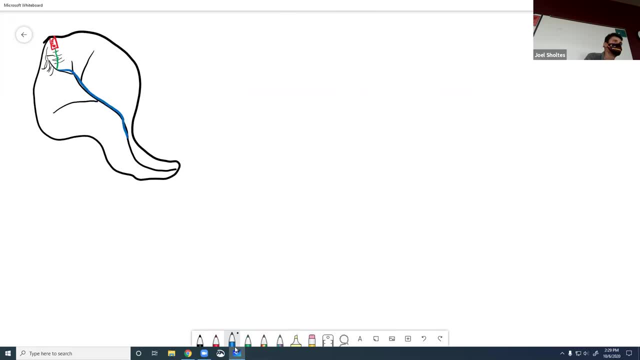 Channel- open channel flow. And obviously this is going to be the longest pathway. It typically doesn't take that long until you meet a channel- Open channel flow. I like that Open channel flow. If you guys end up pursuing hydraulics or hydrology in grad school, you can take a whole class called open channel flow. 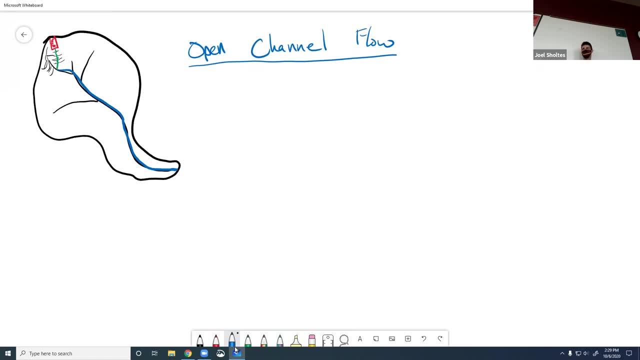 It's beautiful. I took it at Georgia Tech when I was living in Atlanta, just a class And the professor's name was Dr Terry Sturm. He wrote one of the textbooks And he would complain about. he spent all this time writing this textbook. 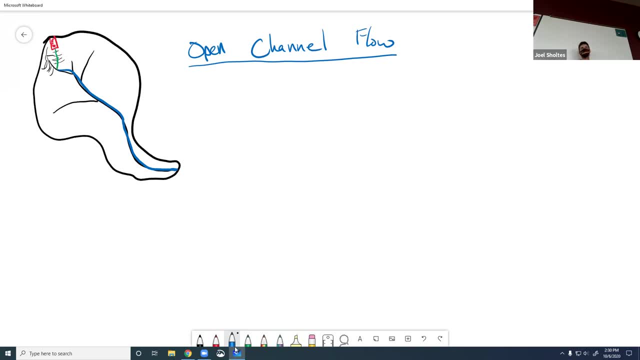 You know it's a huge labor of love. Do you make a lot of money writing textbooks? Do you imagine That's kind of a leading question? I don't know, You don't. You don't make a lot of money writing textbooks. 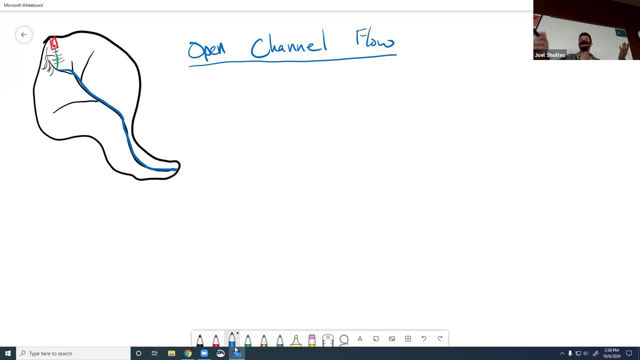 It's not, I don't know. The publisher ends up taking: Textbooks are expensive. You guys know how expensive they are. Publishers end up taking most of the cut. So he's complaining about that in class. Just finish this textbook. 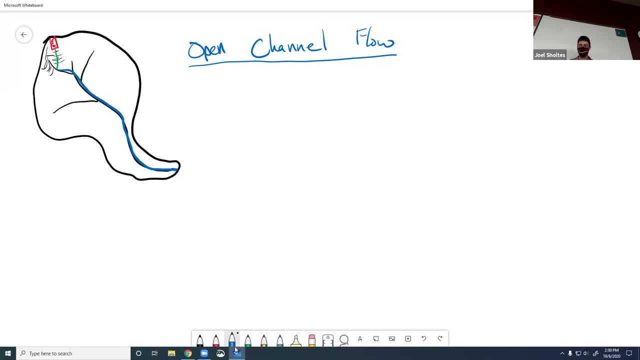 And people are buying all the knockoff versions And I'm sitting there and I got my little paperback version that I got from like Indonesia, You know, like not not made for sale in the US. Sorry, Dr Sturm, I appreciate what you're doing here. 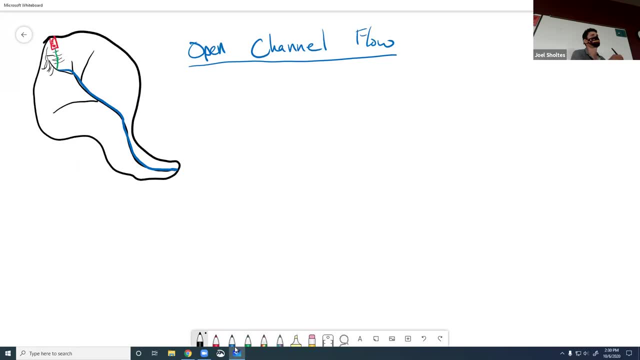 All right. So he's like: this is my textbook Directly to the students. Right, right, right. I don't know if that's legit, but I respect that. He's like no textbook I can really cover what I want to teach. 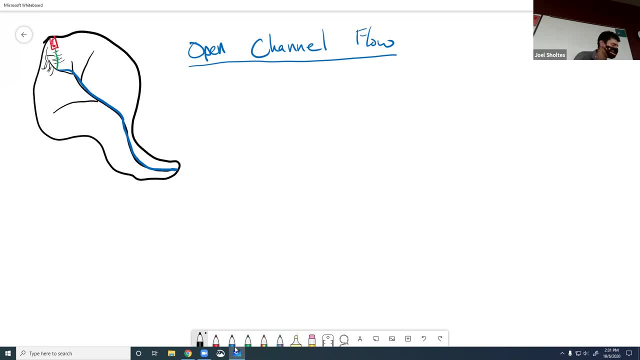 I feel that way about hydrology. Okay, I don't know if I'm going to write a textbook down. So Manning's equation. And now this is Manning's equation in kind of its full form. You'll note that Manning's equation kind of pops up everywhere. 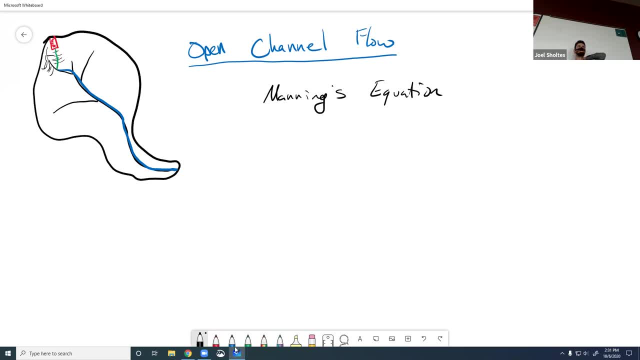 The first two methods that we just covered have Manning's equation embedded in it in some way, shape or form, The coefficient or a simplified version of it. Why do we do that? Because it's around, It's easy. Hydrologists are lazy. 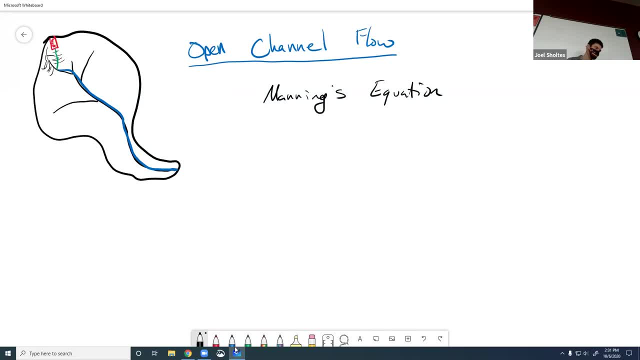 Or hydrology is hard and we kind of need a shorthand to do it. So that's kind of what's behind it. We're estimating all this stuff. So we'll talk about how to kind of be conservative in it all, All right. 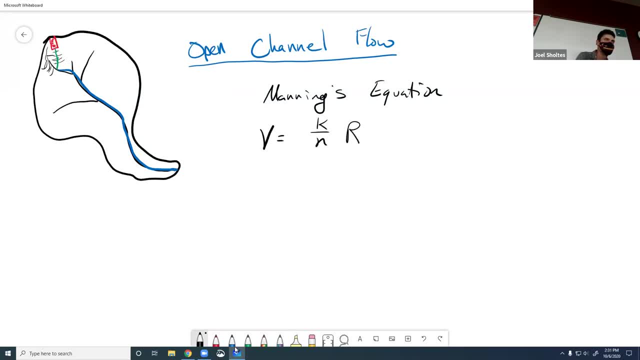 So Manning's equation: V is equal to K over N, R to the two thirds, S to the one half. Does anyone remember what K is from hydraulics? It's a coefficient Yep. So one for metric and 1.49 for British gravitational. 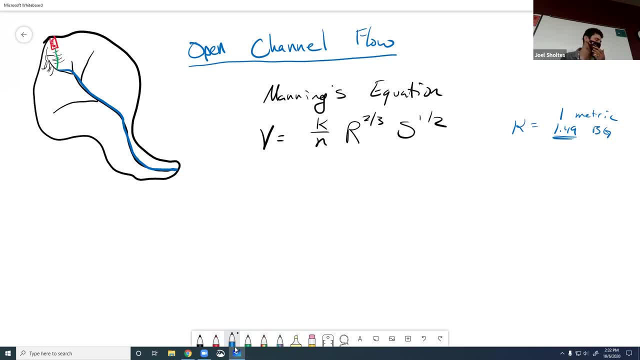 So we're going to be in. you know, US units, British gravitational units, So 1.49.. This is our Manning's coefficient. Does anyone remember what R is? What's that? Did you say it No? 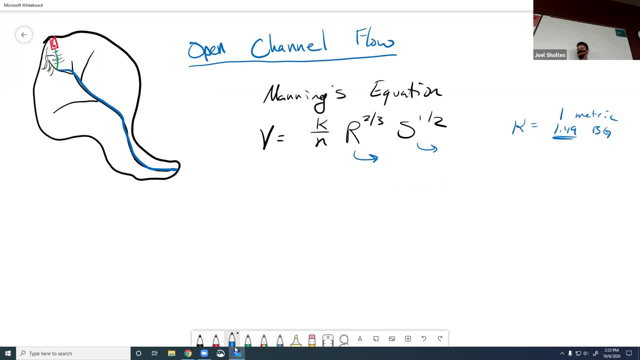 Yeah, Oh, good question. Yeah, Reynolds number. No, that's pipe flow. There's Reynolds for open channel, but that's a little more complex. It's hydraulic radius. Yeah, Jake, Hydraulic radius which is equal to the area over the wetted perimeter. 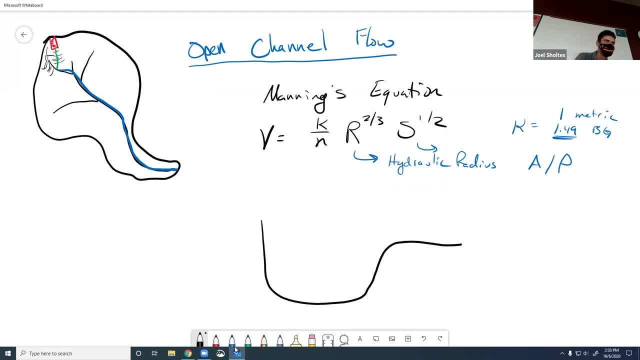 I'll draw a channel for you real quick. So here's a channel. Here's our wetted perimeter And then our area. right, It's just a cross-sectional area of the flow. What's that? Yeah, you know, it's just what's touching. 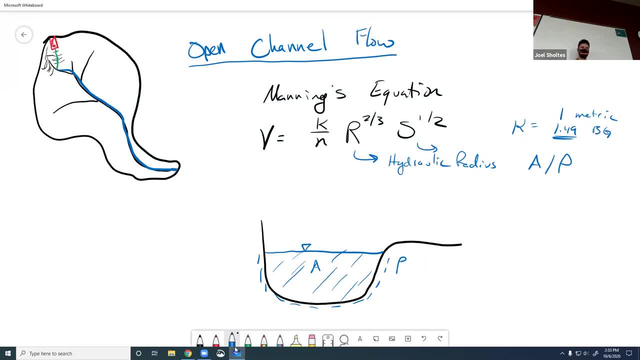 That gets it dragged Like what's touching the edge of the channel, So what could be slowing the water down? And then that's our slope right. So it would just be feet per feet. Okay, So for natural channels N is going to be different than what it is on the ground. 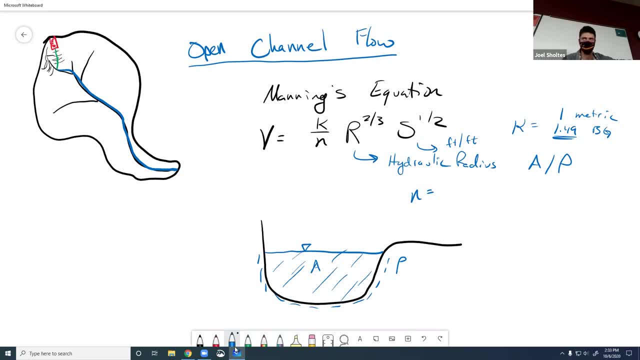 Like if water's flowing on the ground. When you're flowing on the ground, it's much rougher. You got a really tiny flow depth. You got grass, blades, rocks, sticks, all this stuff, So our N is going to be much lower, relatively speaking. 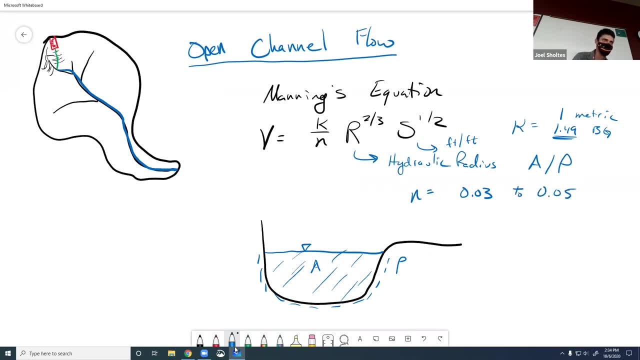 And for natural channels. this is just kind of a very basic range for natural channels. If you're in a conduit, you know stormwater pipe that's different, Different story. You know concrete is going to have a Manning's roughness about 0.013 or something like that for concrete. 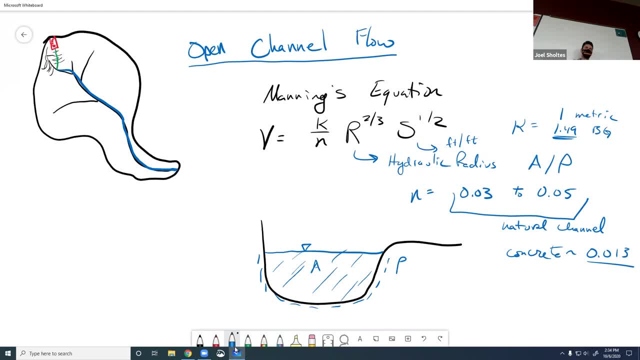 So how do we do this? What like this is kind of a big thing here: Open channel flow. We're trying to calculate the hydrograph, And in order to calculate the hydrograph we need to know all these flow depths. 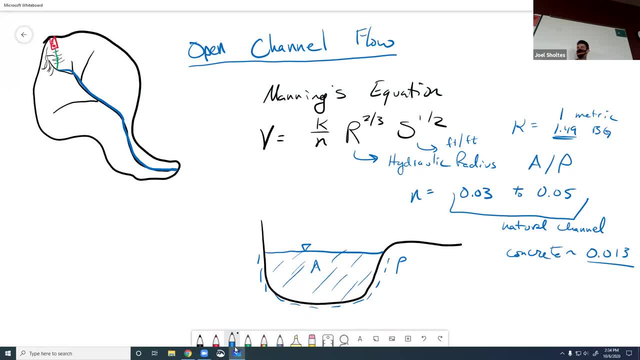 We need to know A, We need to know P And all these things We don't know. We know how much volume we have from the curve number method. We don't actually know the flow rate yet And we're trying to use this method to calculate the flow rate. 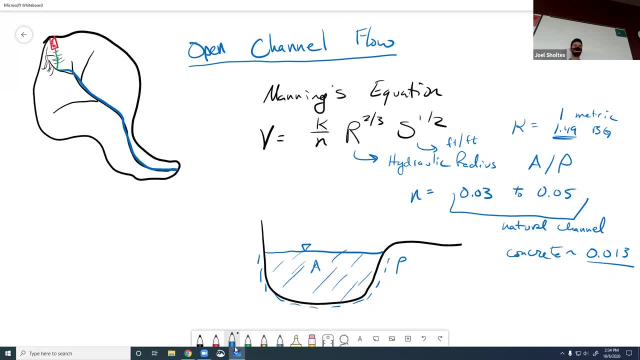 So what you end up doing- and you'll find out in HEC-HMS- is you just make some real basic assumptions. You say, okay, it's a big flood, So I'm going to say the channel is full And I'll set my channel dimensions based on a real estimate of you know what's the channel dimension, maybe at midway in that watershed. 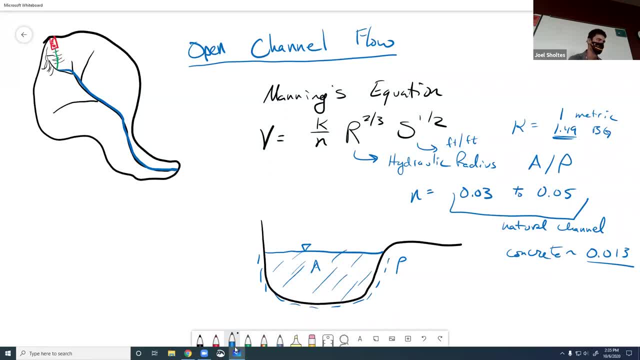 I'm not going to like look at how it changes From a first order to a second order and on down. You could do that. That would just be a little more complicated for your reaches. And this is where this comes into play as well- is, when you parametrize your reaches is you have to figure out what's the width of the channel? 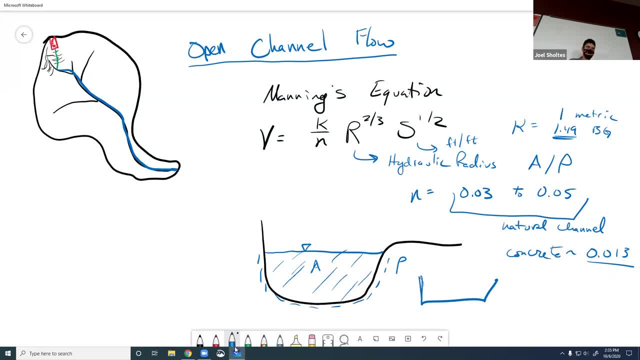 I'm going to call it a trapezoid. right, We'll make it simple. We'll call it a trapezoid. It's got a width, It's got some sort of depth and, you know, maybe a one-to-one slope or something like that. 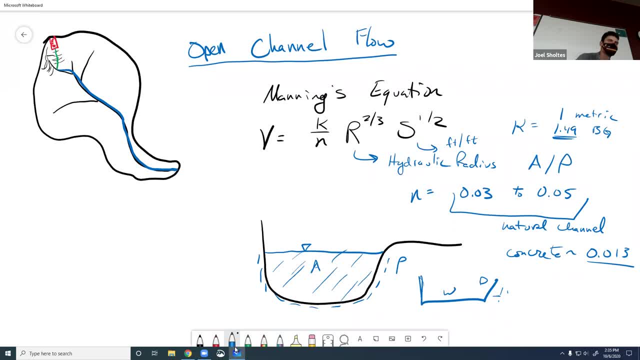 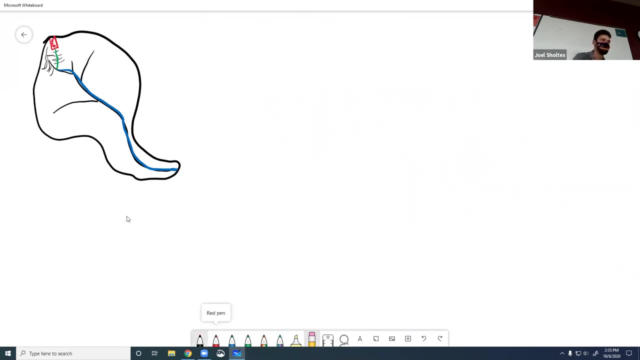 So you really simplify the system and you make some big assumptions, And that, my friends, is how we calculate time of concentration. So I'll just remind you that time of concentration is- well, that was velocity, right? So we have to go from velocity to time in hours. 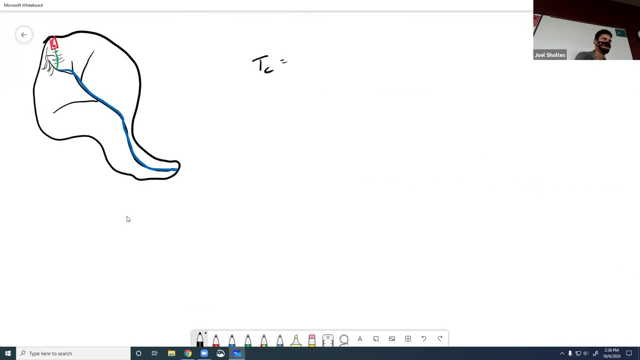 But we already learned that. So time of concentration again is time of sheet flow plus time of shallow concentrated flow, Plus time of water flowing in the channel. And if we want to draw a real simple hydrograph, a triangular one, And we have our little hydrograph, our rainfall depth, right here. 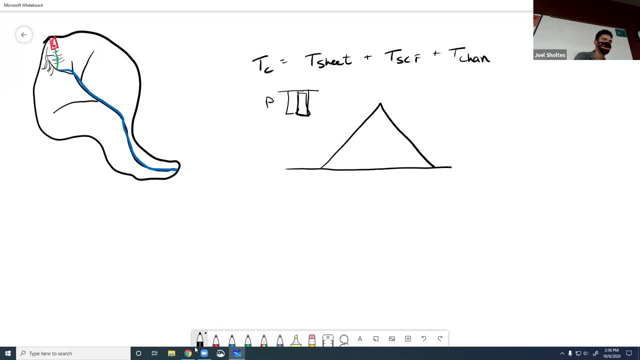 So this is just some, you know, precipitation, And this is Q and our time, And we want to know how long it takes to get from the centroid of that rainfall to our peak, which is our lag time. Well, we can say that our lag time is equal to 0.6 times the time of concentration. 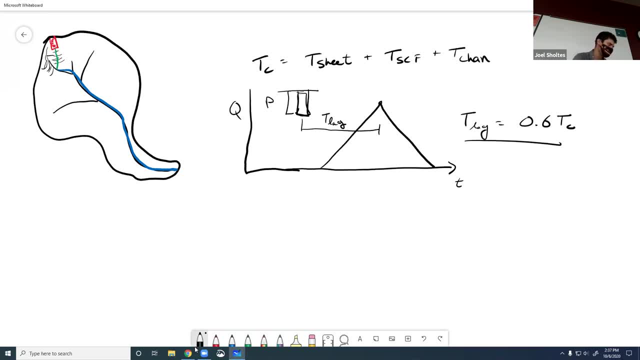 A big, a big estimate, But it's what we use. So what have we done so far? Let's do a quick review. Yeah, Yeah, Right here. Yeah, so this is just a kind of a convention. Let me just erase that. 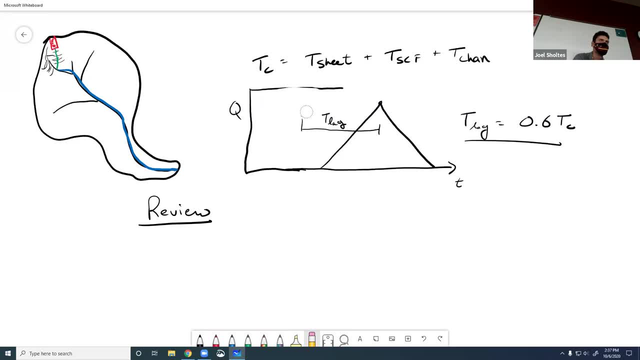 I'll draw a little better for you. Yeah, This is a convention that people use to draw precipitation Or the The top of the graph. And again, this is just a kind of a I don't know what you call it. 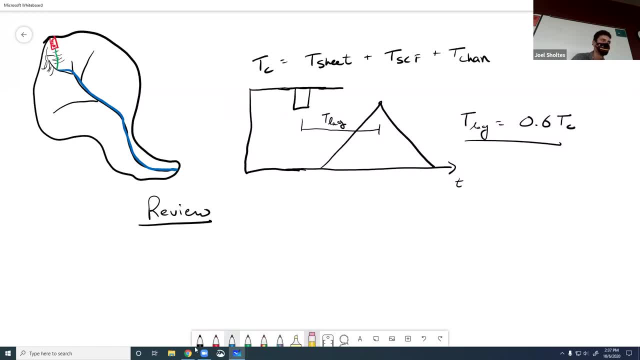 I don't know how you're going to call it, But you can use the top of the graph, So this would be. So this is just a kind of a A high-beam graph On the same access or the same kind of chart. 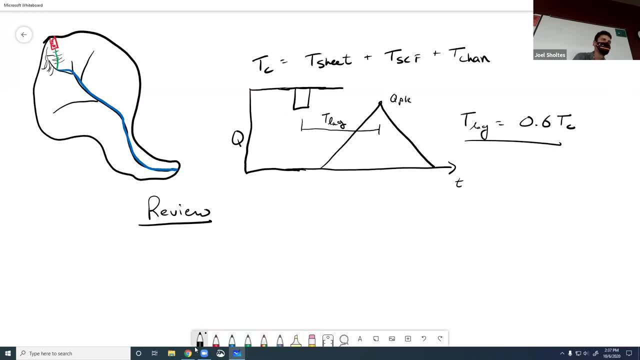 As the hydrograph. So if we have Q right here, Or hydrograph right, And this is our Q peak, This would be- And I'll just kind of Like draw it right here- This would be precipitation. So this is CFS. 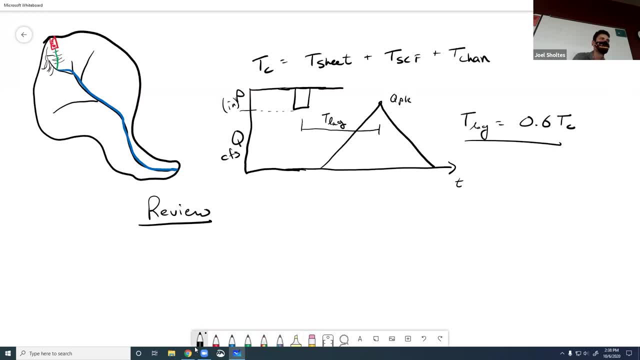 This is precipitation in inches, And I'm just drawing this on a graph That's upside down. I don't want to go too deep into it. I could. I could draw it right here, Right, And just have a secondary access. but I'm drawing it here because this is kind of a convention that people use. you know, maybe you can think about as rain falling from the sky, Right? 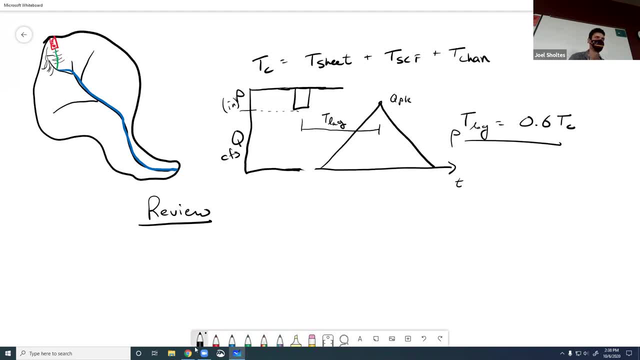 It's just a little confusing because it's going down, Yeah, yeah, And this particular parameter, the lag time, is between the centroid of your rainfall. I'm drawing it simply. I could. I could draw this if it were like a- I hate a graph. Right, The centroid would be somewhere over here. 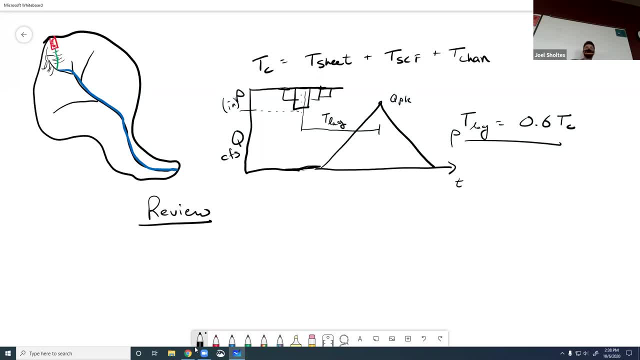 Not the peak, the centroid, The precipitation center, The centroid. How do you calculate the centroid? I'm not going to get into that. It's not like we're going to keep it simple, Yeah, So that's why. that's why I've been drawing just one little bar, So it's simple to visualize. 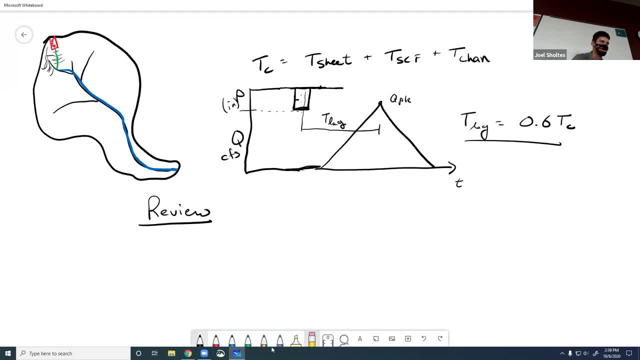 So let's take a look back at our kind of runoff modeling journey here. We started with the curve number method And what did we estimate with the curve number method, Val, Remember, we had the numbers for land cover. Yeah Yeah, We put some rainfall on the lands and then, based on the curve number and that equation, we estimated. 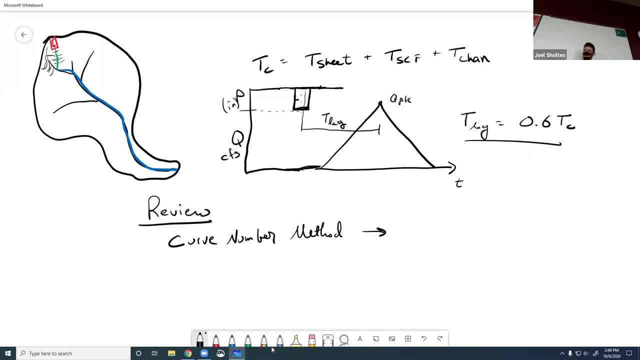 The what. That's okay, Christian, do you remember? Yeah, So runoff. And that equation said Q, it's just the nomenclature they use, but it's the runoff volume. You know that equation was in inches, right? And then we do depth times, area to get volume.